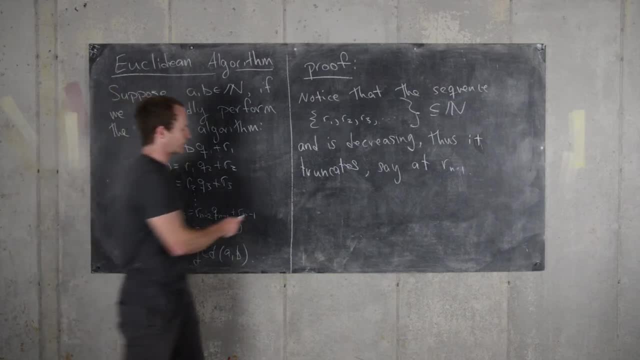 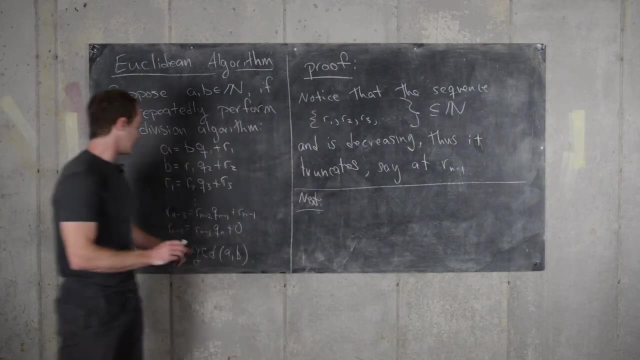 okay, good. so the next thing we need to prove. so the next thing we need to prove is that this last positive remainder is actually the GCD. so we'll first prove that it's a CD, that is, it's a common divisor, and then we'll show that it's. 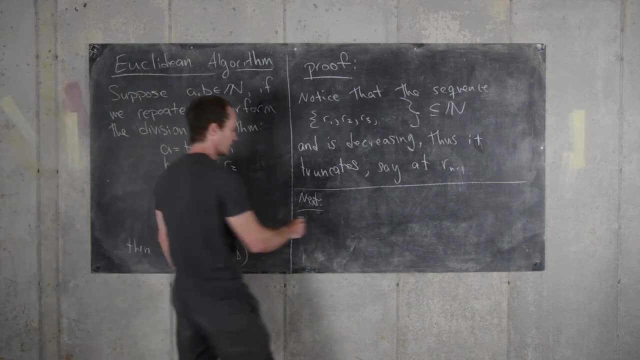 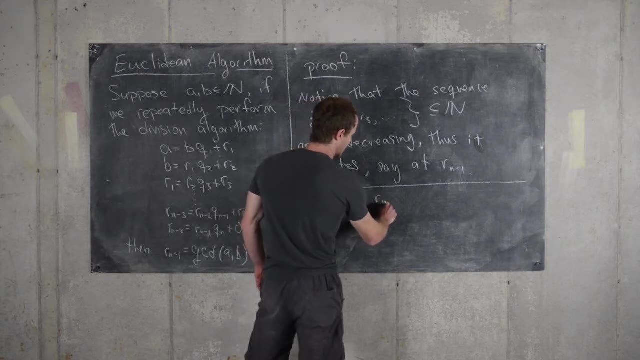 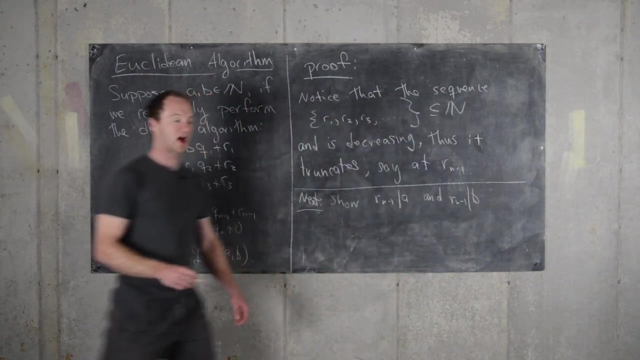 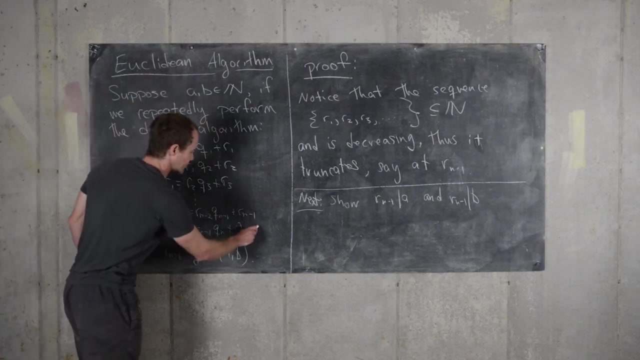 the greatest such common divisor. so let's make this claim: we're going to show that R? n minus 1 divides A and R? n minus 1 divides B. so it's a common divisor. and how can we do that? so this equation, so this equation right here, shows that R n minus 1. 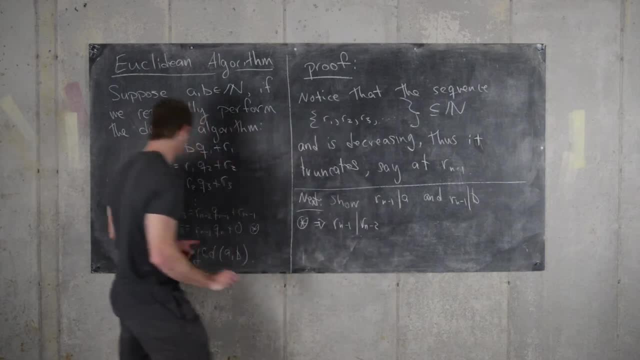 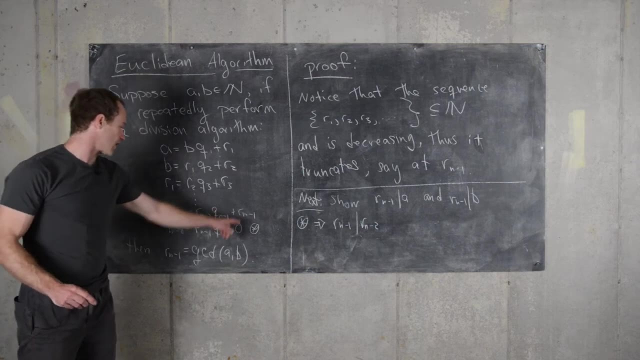 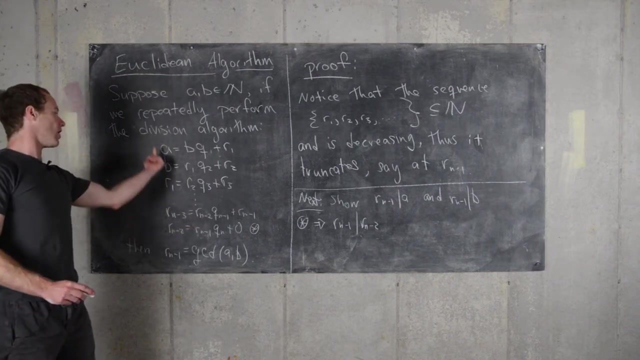 divides R n minus 2, and then, moving up from there, we see that that will show that R n minus 1 divides R n minus 1 and R n minus 2, so it has to divide R n minus 3 and then, all the way to the top, it will divide A and B. so these will all. 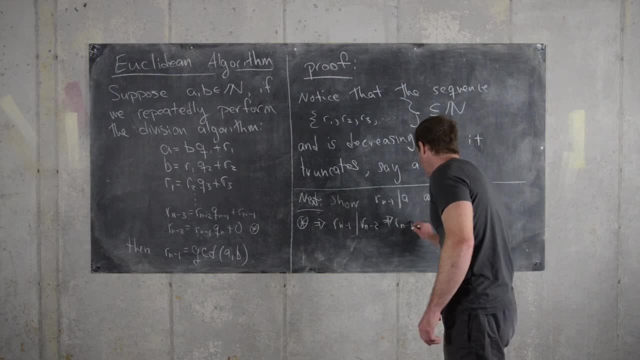 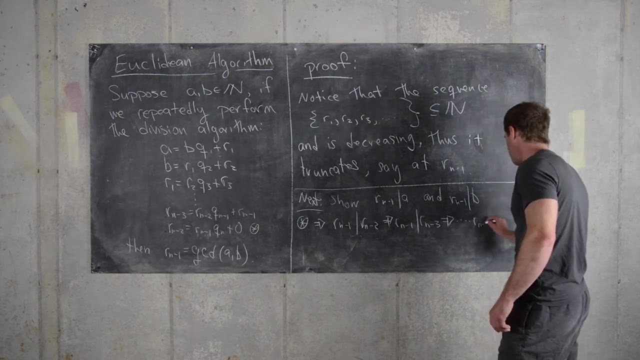 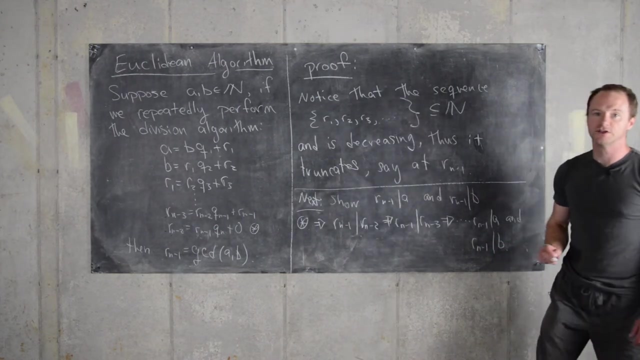 fall from each other. so this means R n minus 1 divides R n minus 3, which implies that dot that R n minus 1 divides A and R n minus 1 divides B. okay, good, so that means this last nonzero remainder is a common divisor of A and B, so I'll clean. 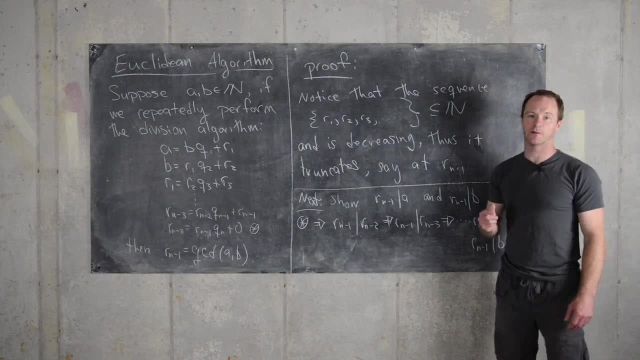 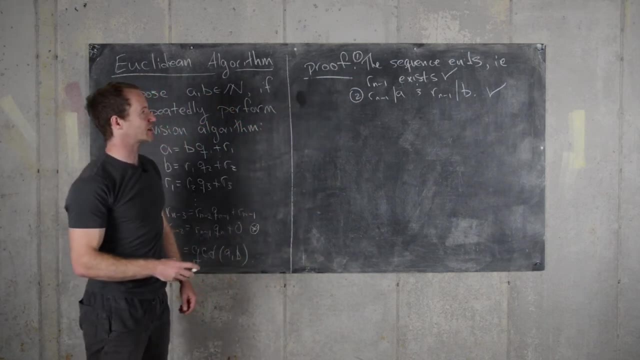 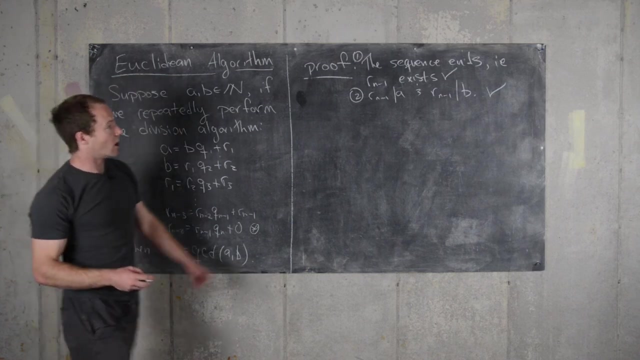 up the board and then we'll prove that it's the greatest such common divisor. ok, so now we're ready to finish off the proof. so I've reminded ourselves that this sequence of remainders actually ends. in other words, this R n minus 1 exists, the last non-zero remainder. And also we've proven that Rn-1 is a common divisor of A and B. 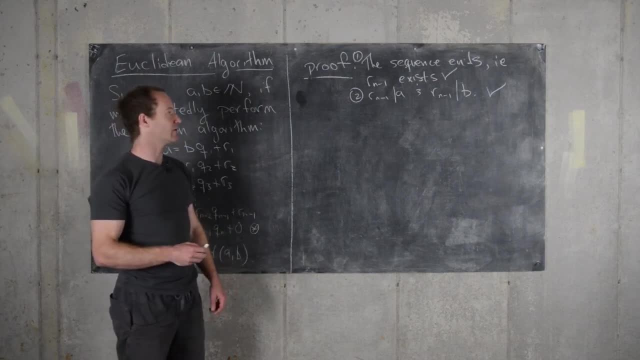 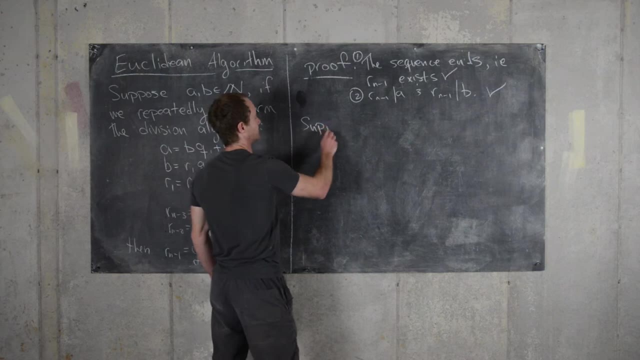 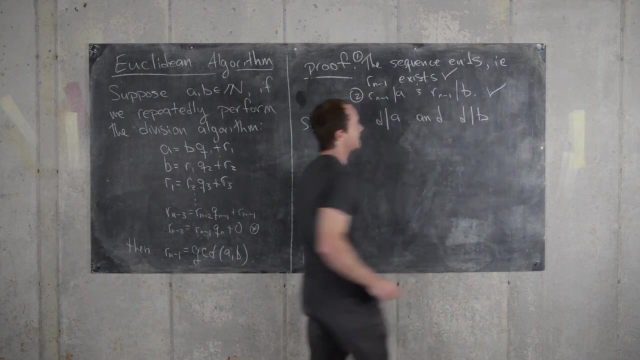 That is, it divides A and it divides B. So now we want to show that it's in fact the greatest common divisor. So how can we do that? Well, let's suppose that D divides A and D divides B. In other words, we have another common divisor of A and B And then our goal, which we can put,